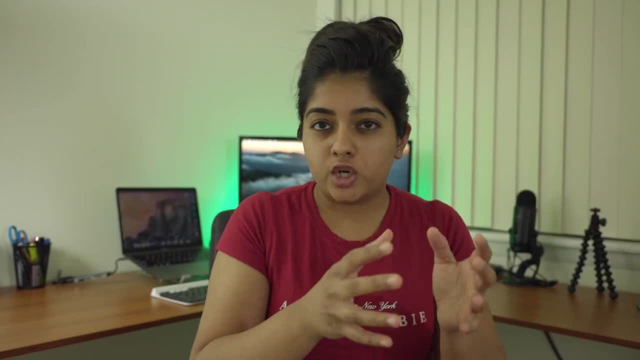 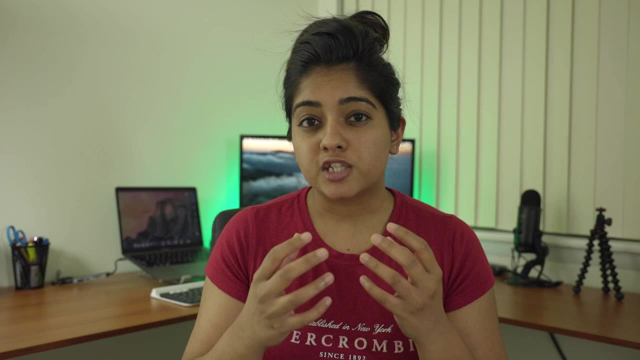 what's wrong with you. Literally, if you're going to go into a doctor's office, you need to find out. any piece of machine or equipment or technology that you use or step into is probably designed by a biomedical engineer, And that's what the core curriculum of this degree involves. So I still 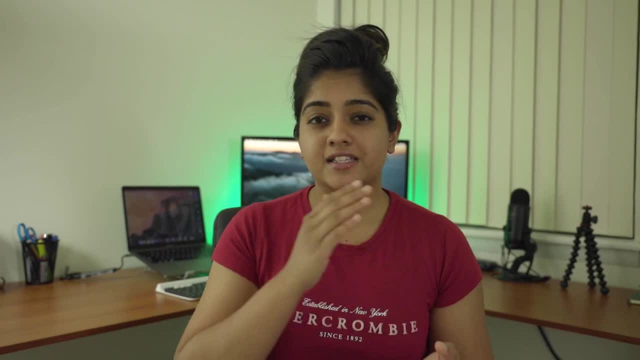 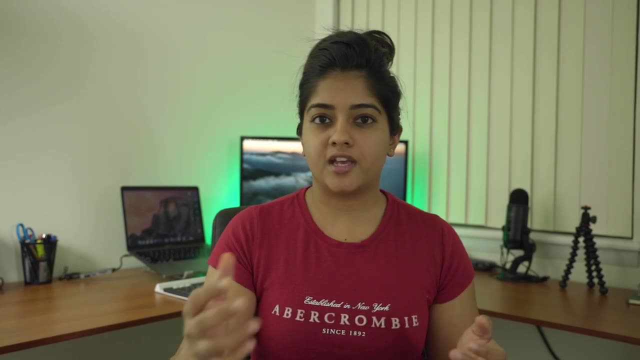 remember when I was studying this degree in my undergrad, I had like separate courses for each machine, Like I literally had a course called ultrasound and its applications, x-rays, neurology. So basically the idea is, I would have to first study about. 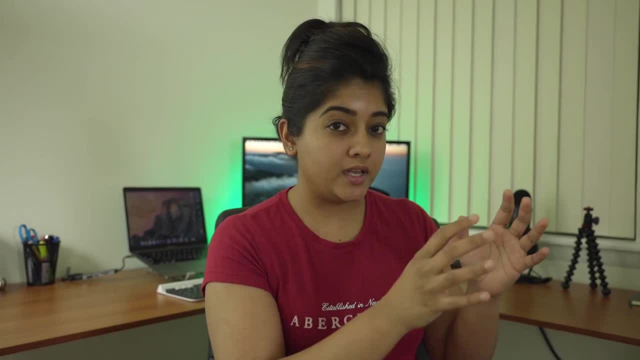 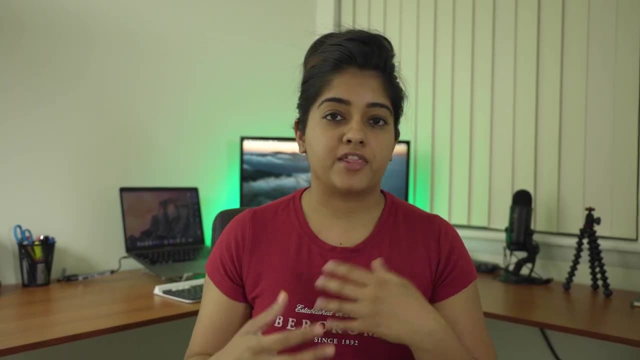 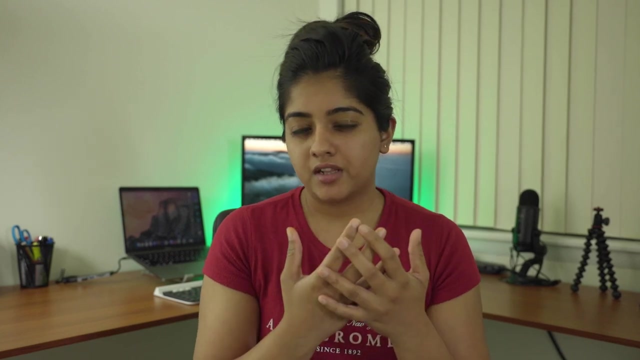 what the disease or what the problem was from like a human anatomy and physiology perspective, And then we would be taught how we can use principles of physics, mathematics, technology basically to solve that problem. So it's really like an intertwined degree, Like I tell a lot of. 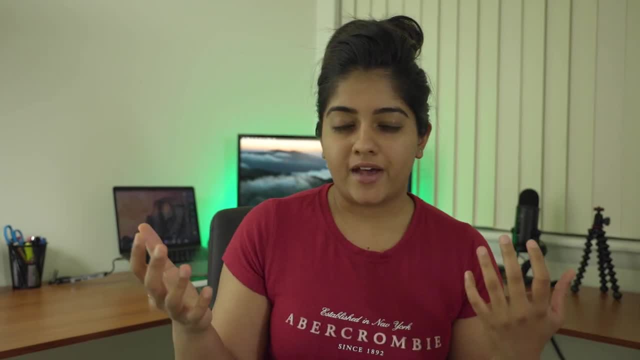 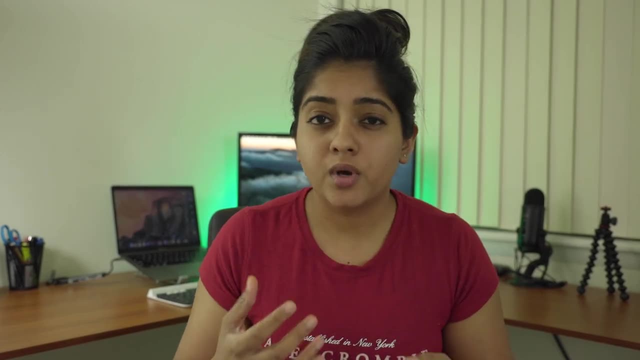 people that if you don't like biology and you don't like math, this is definitely not a degree for you. But if you like both equally, maybe biology even a little bit more than math, you know, this is like a perfect combination of that degree. So that covers the diagnostic part. 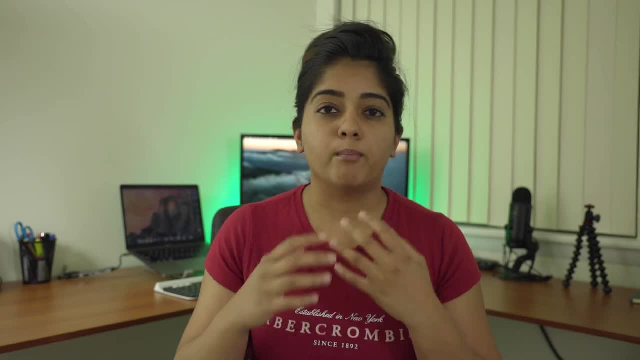 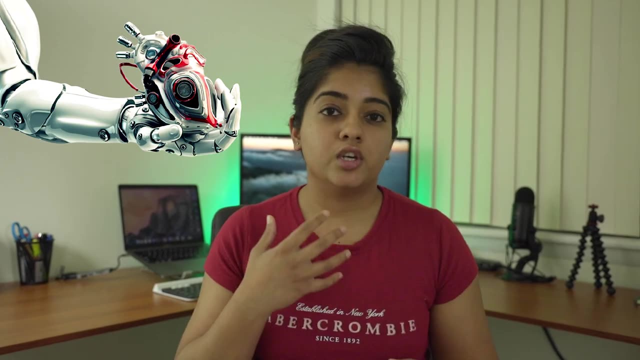 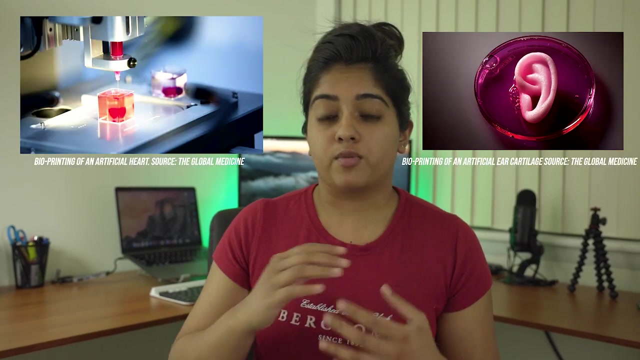 of it. Now, talking about the therapeutic part of it, this involves monitoring the disease. It can be stuff like your artificial organs. Instead of a clean amputation, we, you know, give the ability to a patient to walk. That is all things. to artificial organs There are courses like orthopedics. 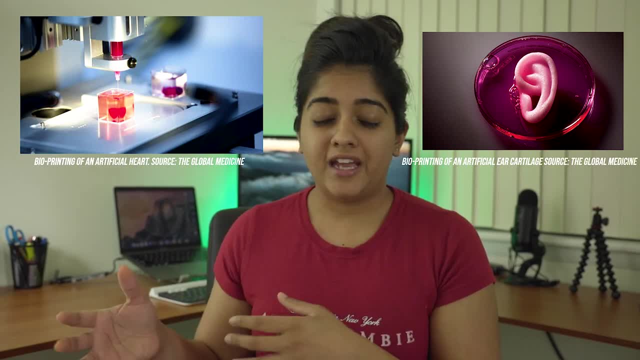 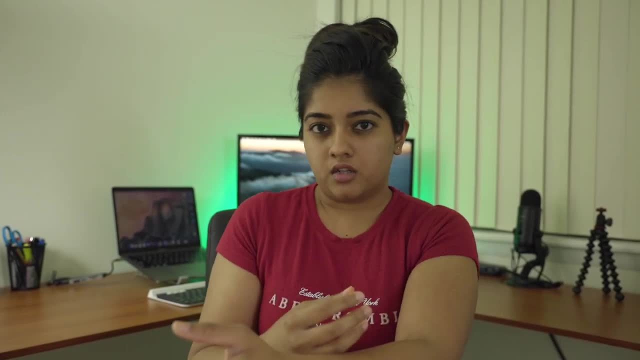 where you extensively study the reaction of your body and how different materials would react to it. Like, think about it. If you're an orthopedic doctor, you have to, you know, do a lot of your own training. if you're cutting open an arm and you just stick like a steel or aluminum or titanium, how do you? 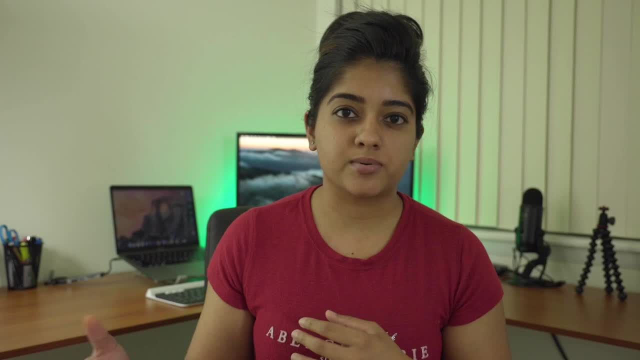 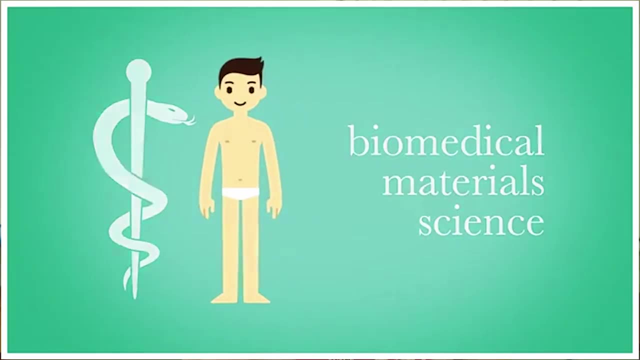 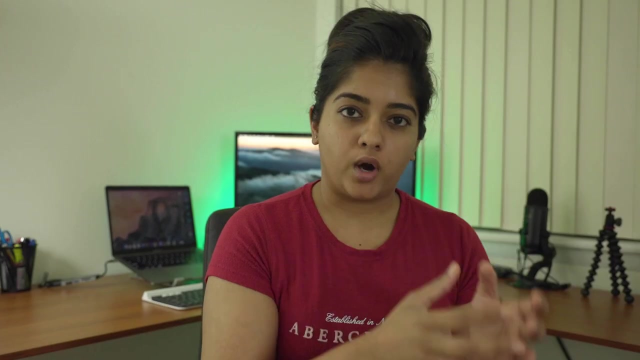 know that your body's not going to reject that foreign piece of substance. essentially, what your body's going to do- and this happens a lot, we- we literally studied this in biomaterials endlessly- is you. there's something called biocompatibility, where you need to study if your body will treat. 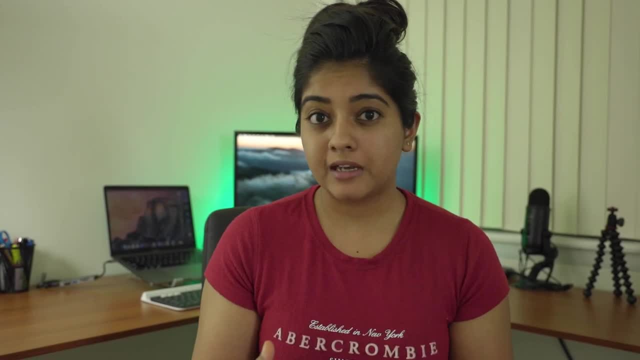 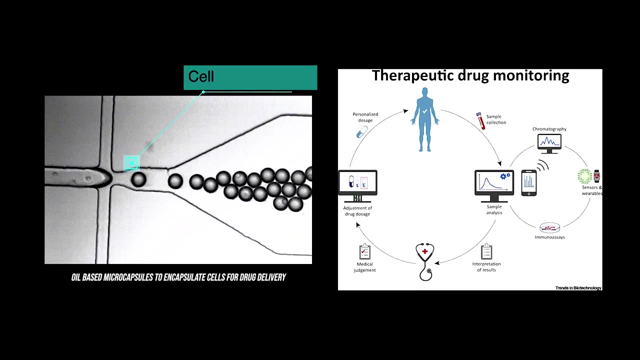 any foreign substance as like an attack. so if it does that, it will start rejecting that and essentially your body will start shutting down. but other things that are included in therapeutics involve stuff like drug delivery systems. um, all of your pills that you take, like, have you ever? 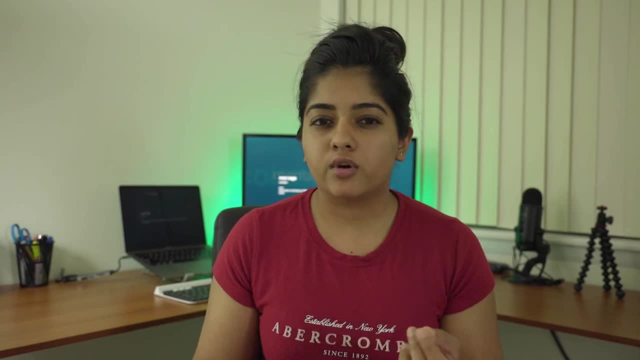 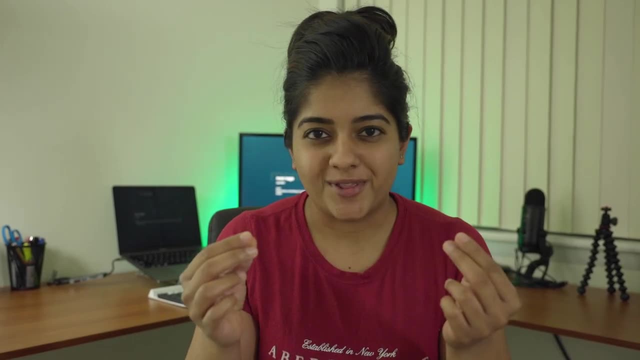 stopped to think about what it's actually doing. remember you know how some tablets are just like tiny and round, but then some are like capsules. um, i don't know if you guys did this, but when i was a kid, i'd always like open those capsules up to see what's inside. it would always be a powder. i never. 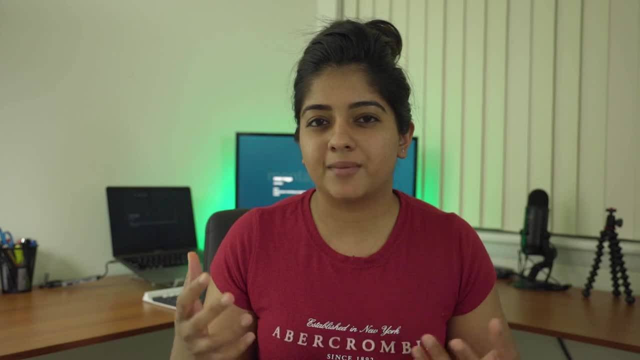 really understood what it was and i never really understood what it was and i never really understood it and i never really understood what it was and i never really understood what it was and i never really understood the point of the capsule that i'm like, you know. i could have just taken the powder it. 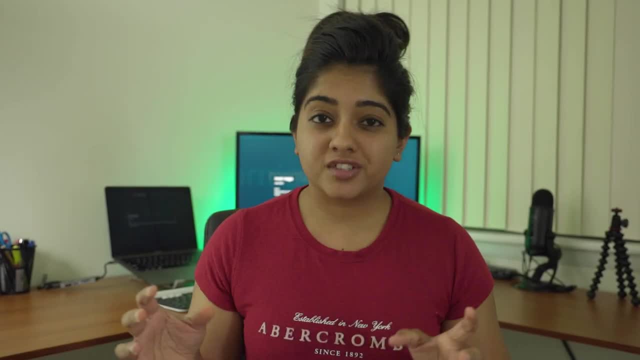 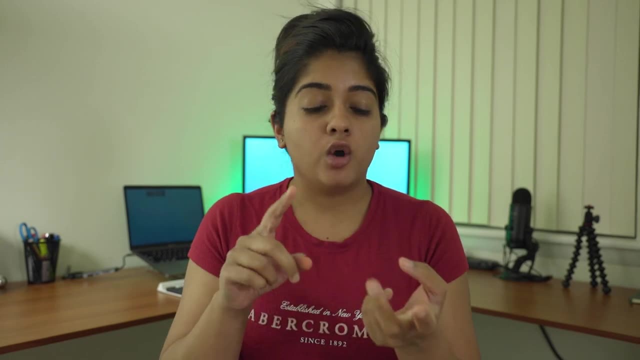 would have been smaller anyway. that is the whole drug. so, basically understanding how you could effectively deliver that drug into your body, what's the fastest way, what's the safest way, and is there a way we can improve this technique? i know that there are a lot of doctors who 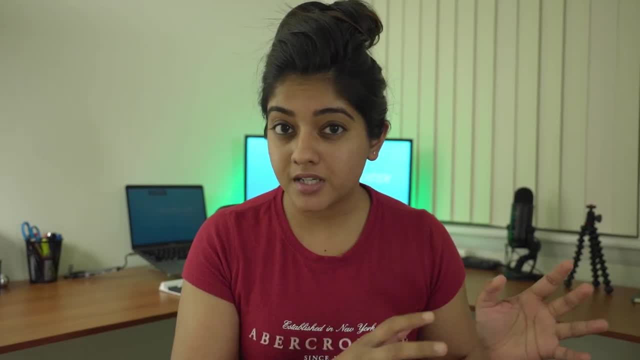 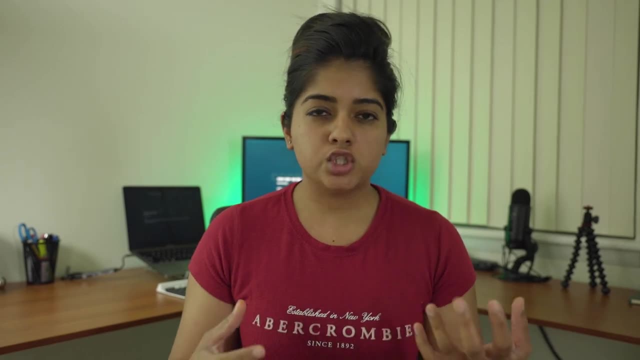 eventually go into research, and i'm not saying that they're not capable of doing this, but the field of biomedical engineering is precisely, if you're interested in doing this. so, in short, if i had to summarize this field, it's basically that you you're not a doctor, but 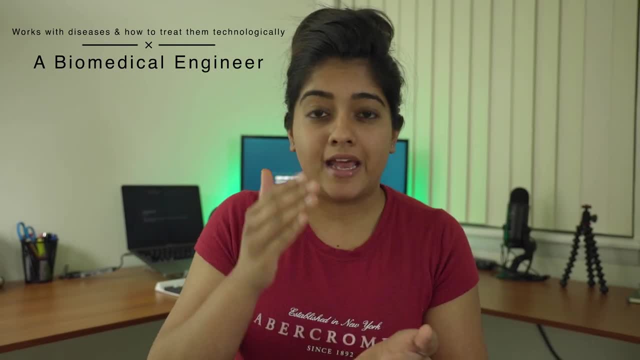 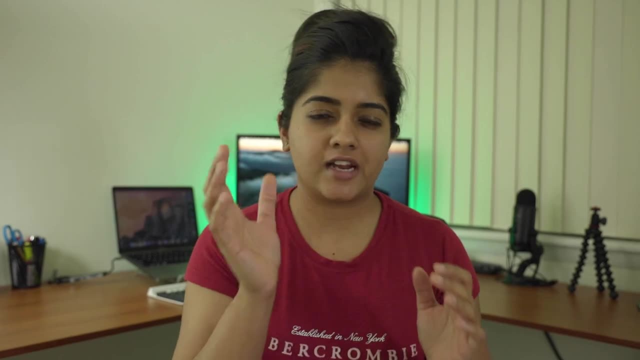 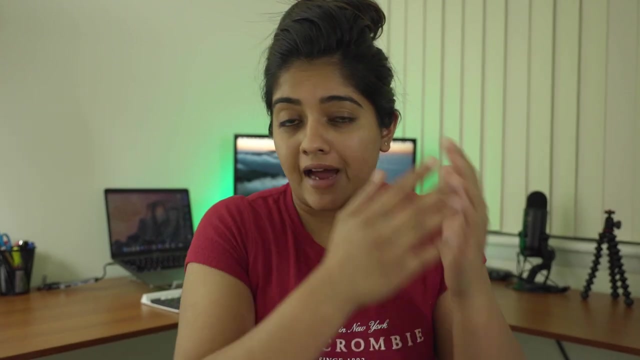 you're very well working with diseases and how to treat them. so i basically spoke about the broad areas of you know biomedical engineering and from everything that i've spoken up till now, you guys probably have an idea that this field is pretty elaborate. there are so many routes you can. 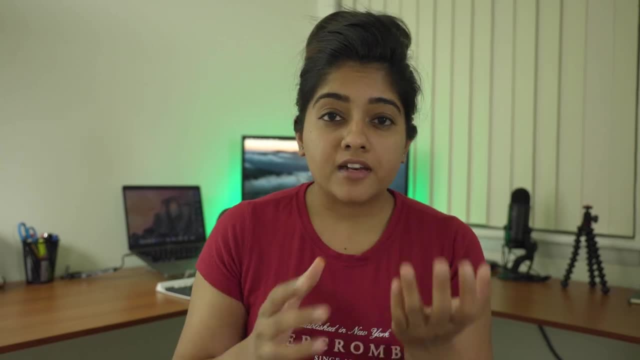 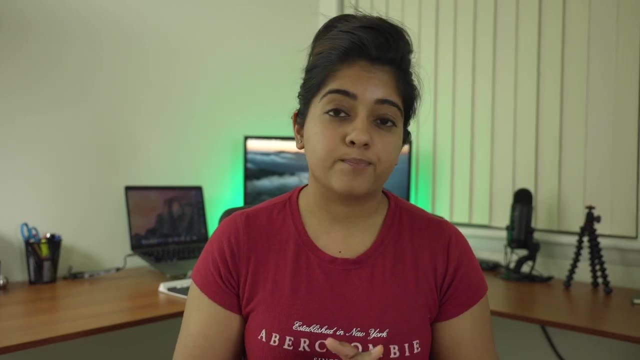 specialize in and shape your career that way. now, with that in mind, i want to go over some of the specializations that you can do if you do decide to go into biomedical engineering- not not. the easiest way to remember this is: you can add bio in front of basically any engineering discipline. 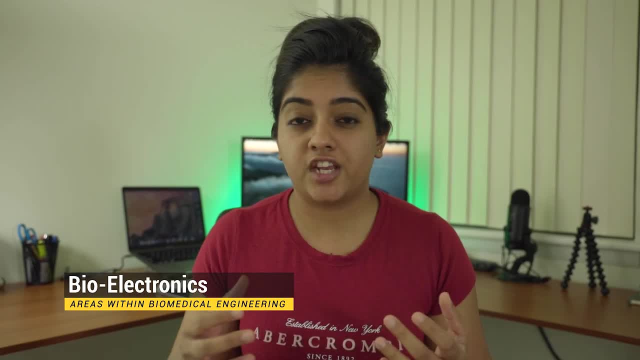 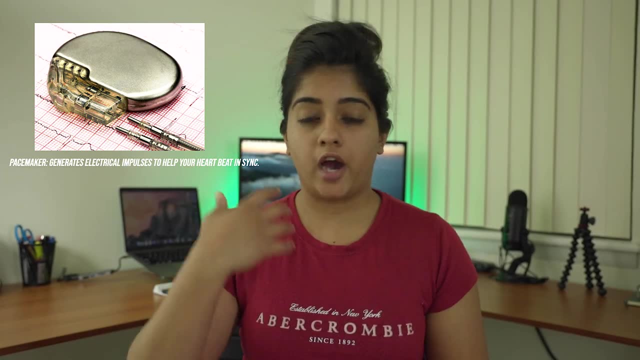 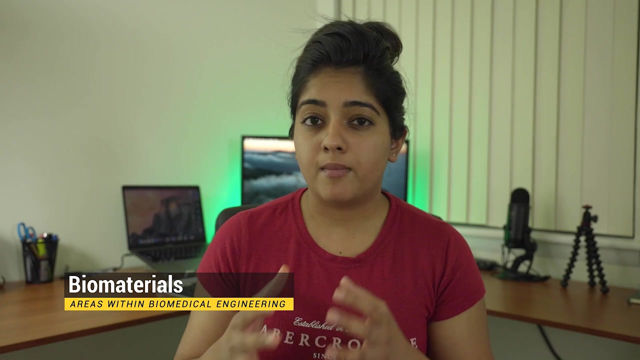 there are bioelectronics, like, for example, think about designing, you know, a chip that you could insert underneath your skin that would constantly read your entire body's like, um, you know, vitals. that's bioelectronics. there's biomaterials, where, again, you study about how different 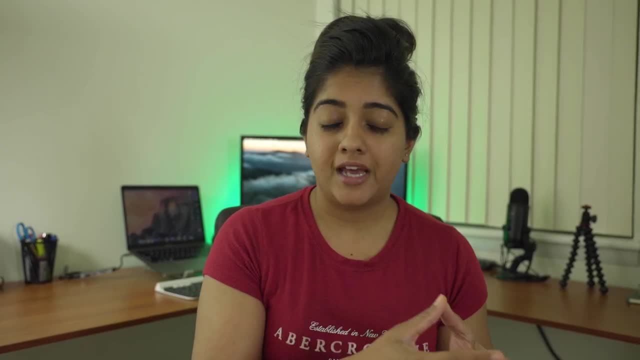 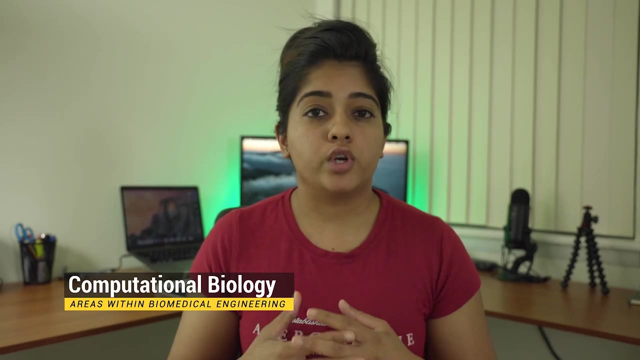 substances, foreign substances- react with your body and what's biocompatible, what your body is okay with and what it really doesn't like. there's computational biology, where you study a lot about how you can effectively analyze the data and what what's the most important information you can get. 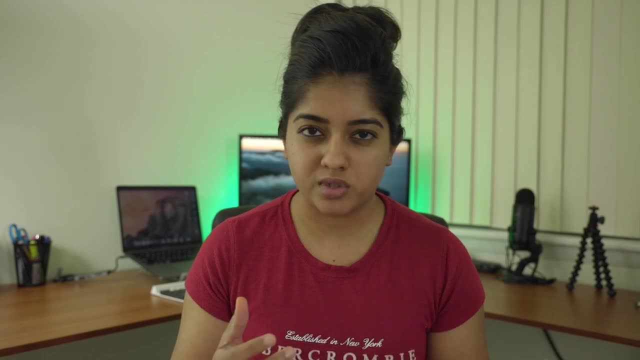 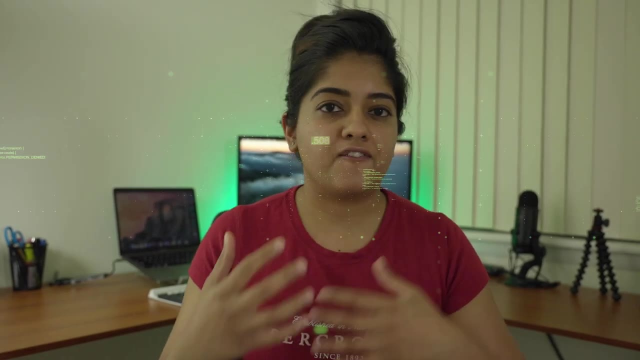 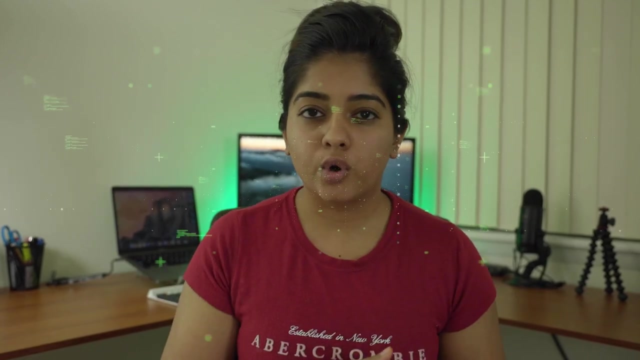 out of it. now think about it. an x-ray scan is pretty much useless if someone doesn't know how to read it. right. that is all computation biology. can you? can we make things faster if a computer were to do it? there aren't enough doctors available to read the scan. can we just run it through a matlab code? 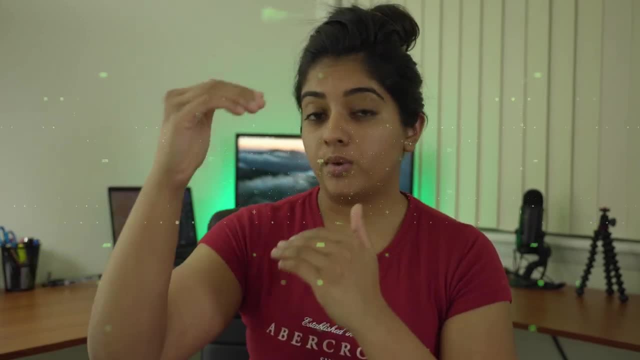 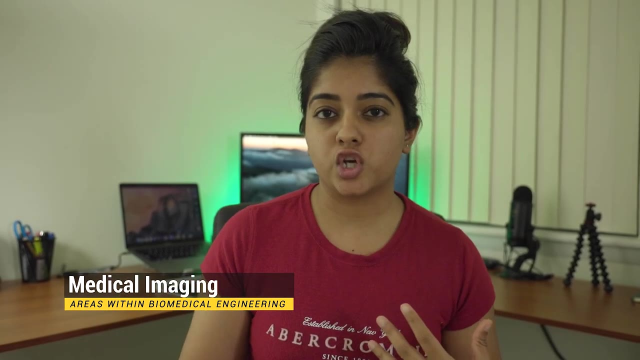 where the output of that code would be all the things that we would need to know. there's medical engineering as a whole separate discipline where we precisely think of different ways we can image. is there a better imaging technique apart from x-rays, mris, ct scans, where we can get more? 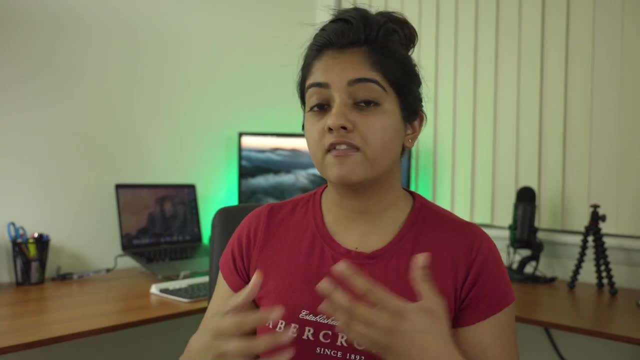 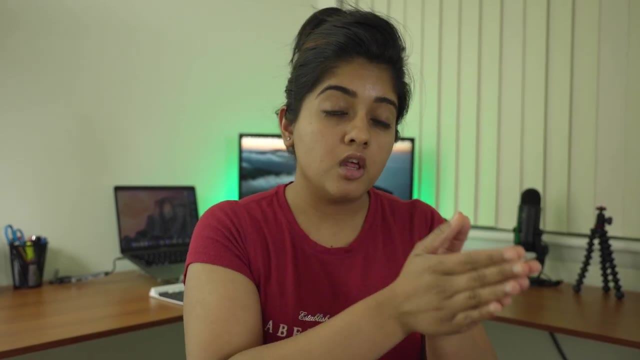 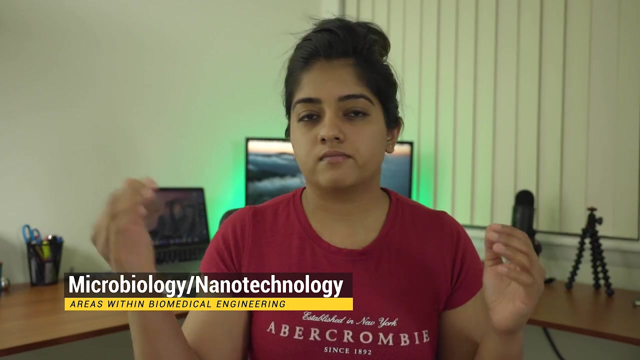 information, so that we don't have to cut open a person, or even if we have to do that, in case of an injury or something, we have the most amount of information available beforehand. and then, of course, there's microbiology. there's in bio, nanotechnology, which again, um, pretty much. 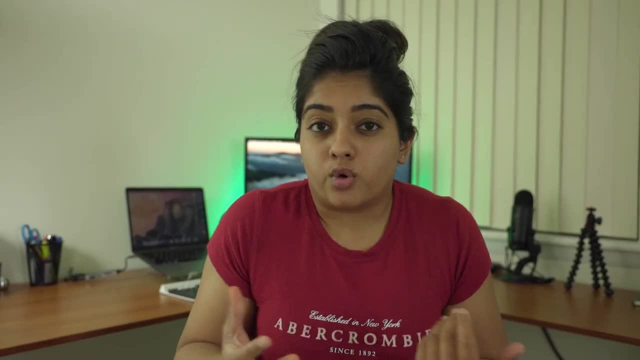 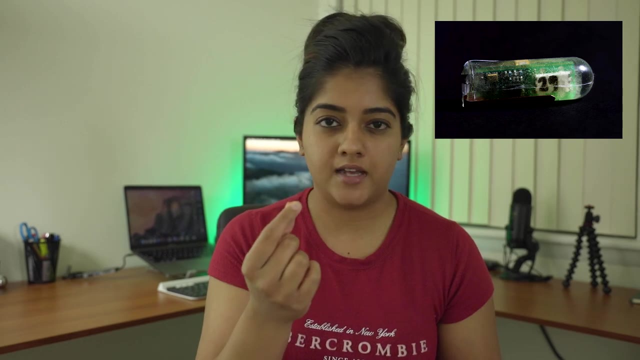 going smaller and smaller onto size. um, is there a faster way we can do this? um, think about something called an electronic pill, like the pill that you actually take as a drug. imagine the same pill, but when you swallow it, what it does is it kind of like turns into. 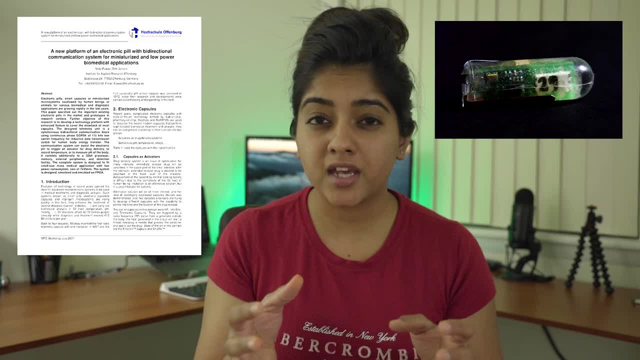 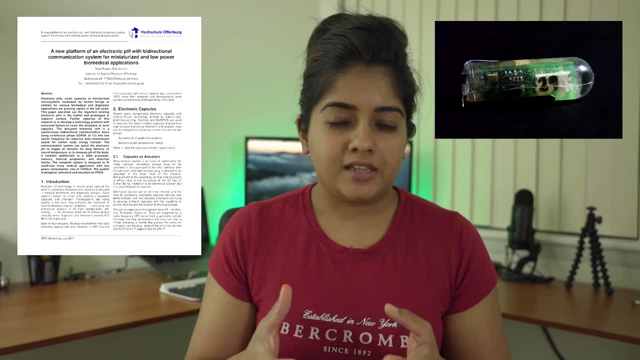 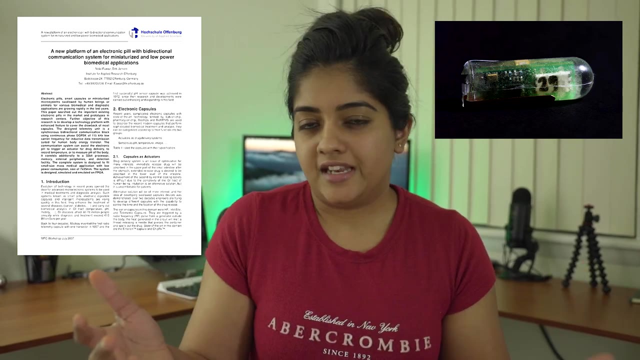 like this alien camera robotic thing. it images your insides, it takes pictures and it conveys that information through a bluetooth device through to your phone. that way it just eliminates the whole need to do laparoscopic surgeries or exploratory um surgeries in any way like that. 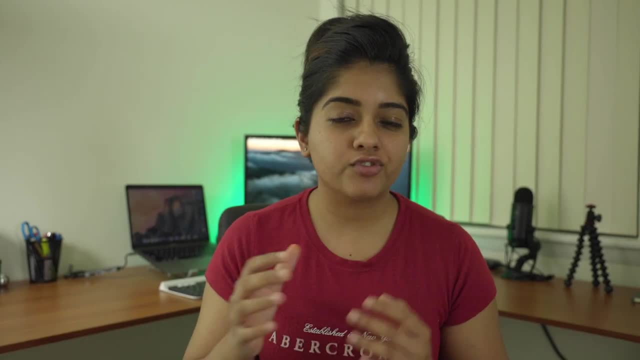 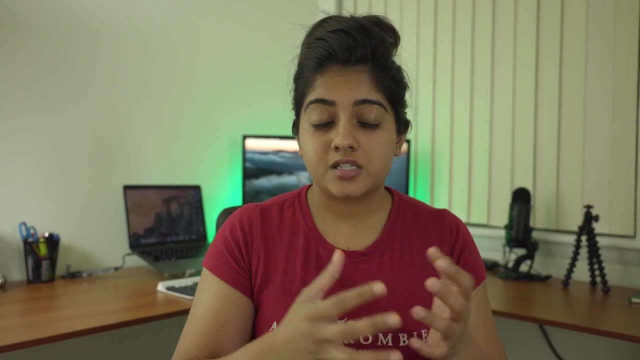 would be so cool, and i'm not just like making this up as i go. most of these things are something most of these things are already being researched upon and, uh, you'll see that this is essentially what you're going to be doing when you're going to be doing a laparoscopic surgery and you're going to 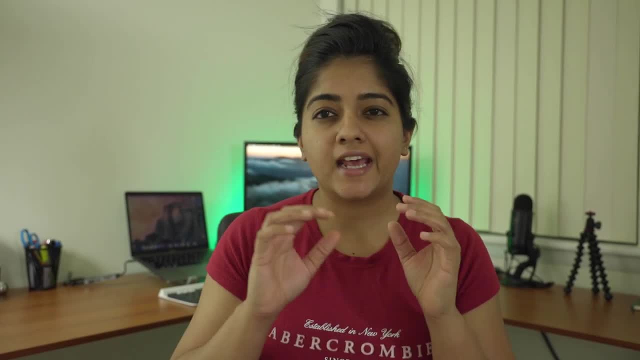 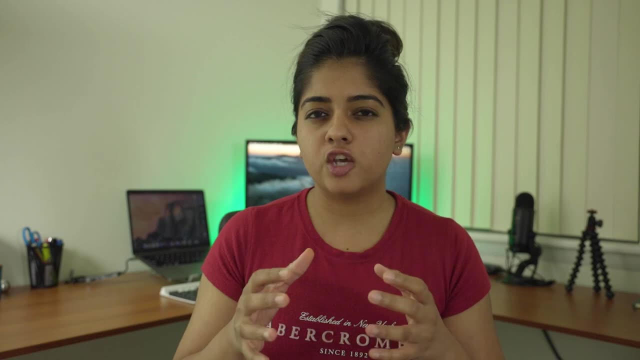 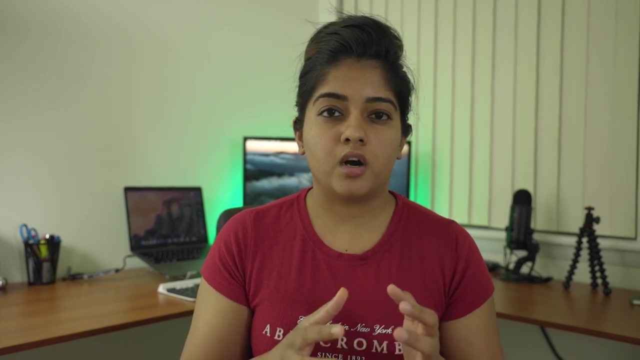 be very careful about what a biomedical engineer would be involved with, and i guess like now is a good time to point out that the cool thing that i like about biomedical engineering is, say, you've completed your undergraduate in something like electronics or mechanical engineering, you can still pursue a career in biomedical engineering because you can take that as a master's level. 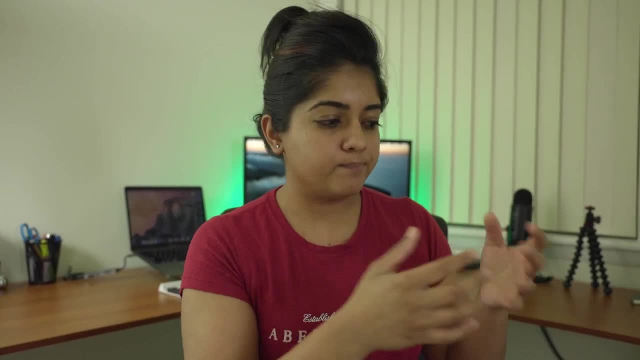 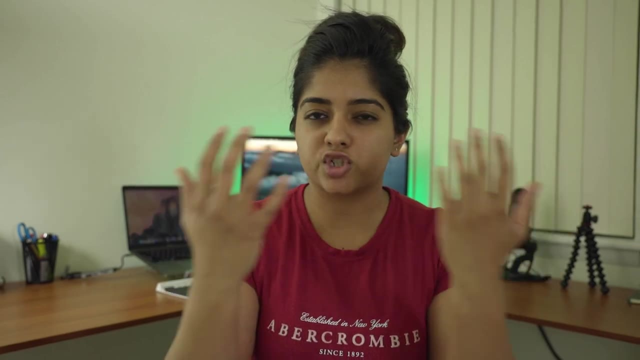 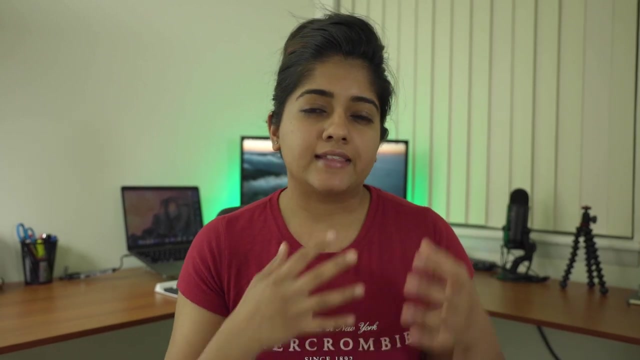 course and use all that knowledge from your undergraduate degree- electronics, mechanics, computer even- and apply that to your course. it's not going to be a waste of time if you into healthcare. So these are just like two disciplines that just nicely fit together. Biomedical engineering goes well with any other field, and that knowledge and that intellectual 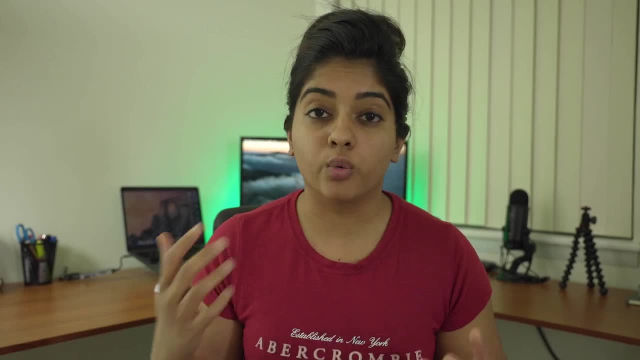 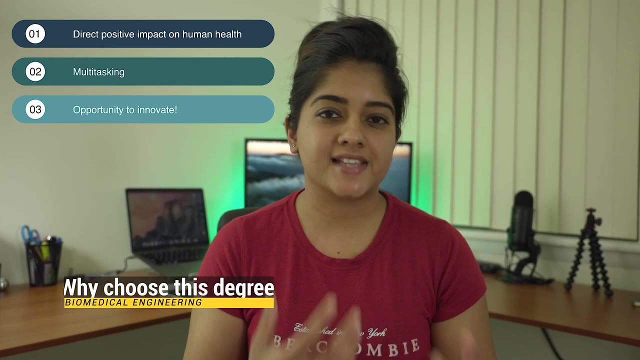 knowledge that you've gained through years of studying does not go waste. The fact that this field has direct positive impact on human health is one of the reasons why I feel it's really satisfying to work in this as a career. The other thing is if you're someone who really enjoys. 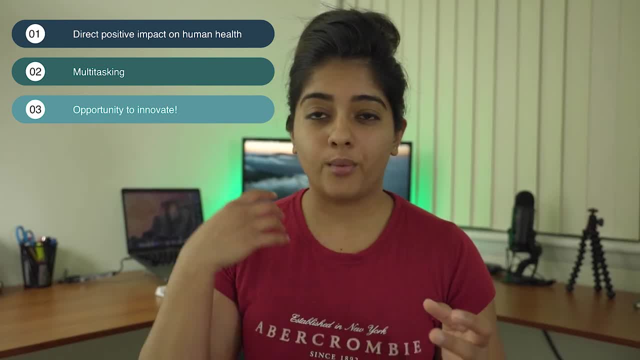 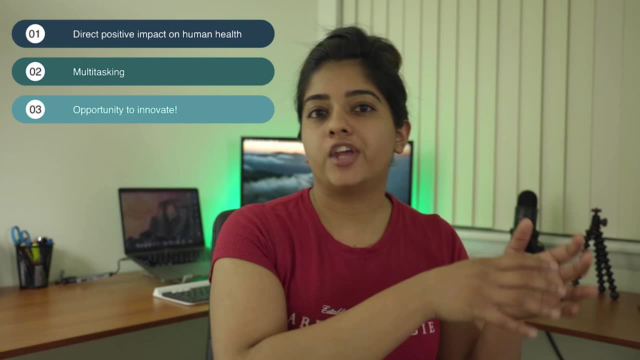 multitasking. this is definitely for you. You're always like learning multiple things, like think about it. in order to learn biomechanics, you first have to learn mechanics and then you can see how you know your body will react to all of these different things. So you're basically learning a. 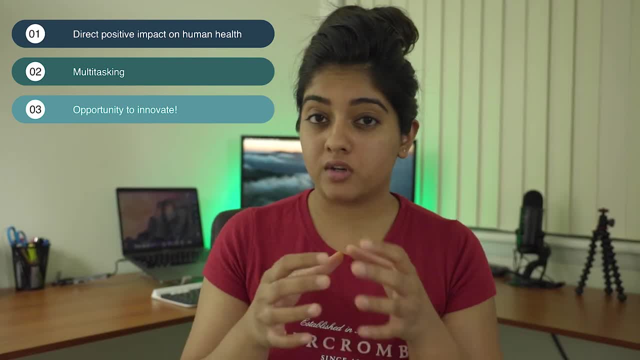 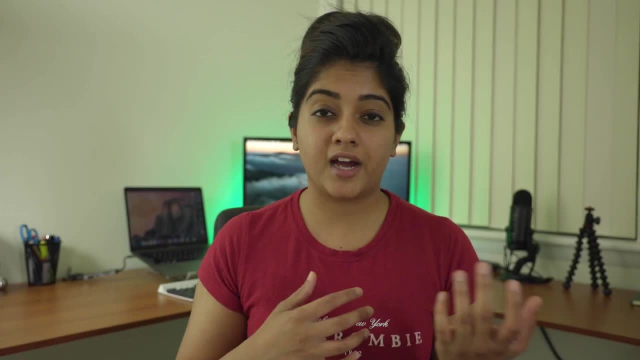 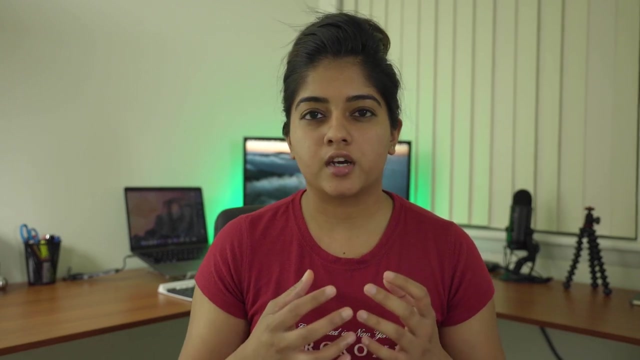 little bit of everything and then trying to apply it to the best possible way, to the human body. And here's the thing you know: nobody knows from the start of their undergraduate degree or high school, or even the end of their undergraduate, With what they want to pursue as a career, and I feel like there's a lot of pressure on us from the 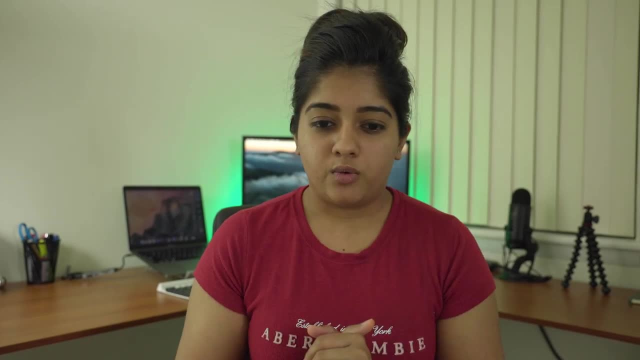 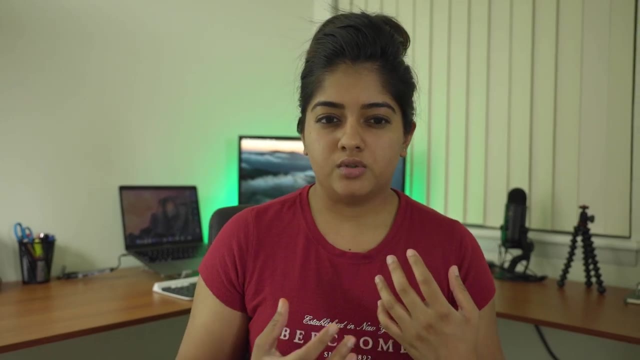 very beginning. You know what do you want to do. Do you have it all figured out? And when I was in undergraduate degree I was so sure that you know the thing that I would like to do and the thing that would be really cool would be to design artificial organs and go into orthopedics. So 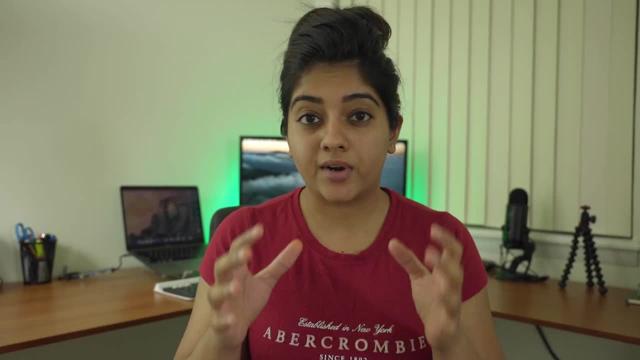 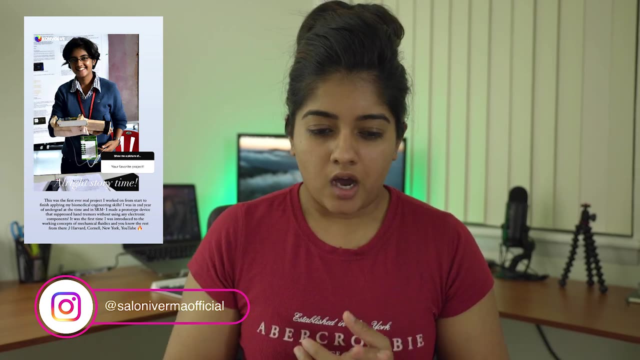 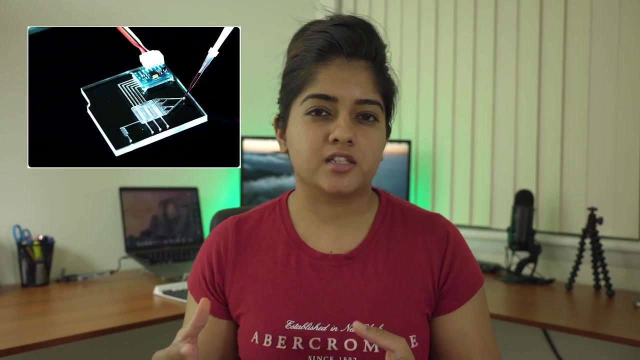 that was my entire focus and I had so many projects revolving around that. A prime example was the prosthetic arm that I built to suppress hand tremors. But as I moved on into my third and my fourth year, I was exposed to this area of microfluidics and 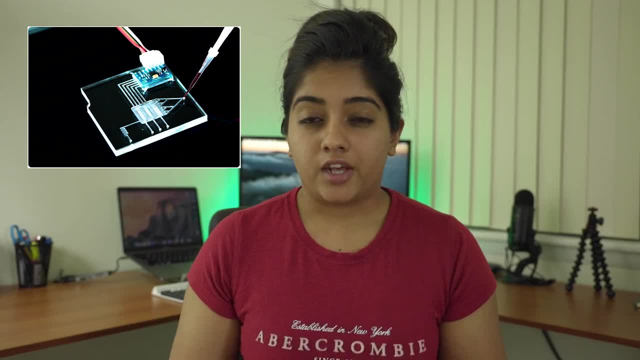 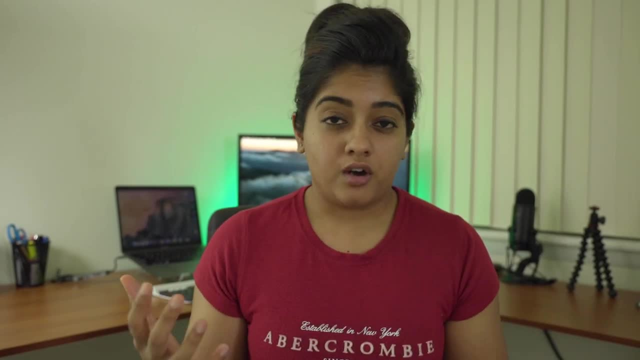 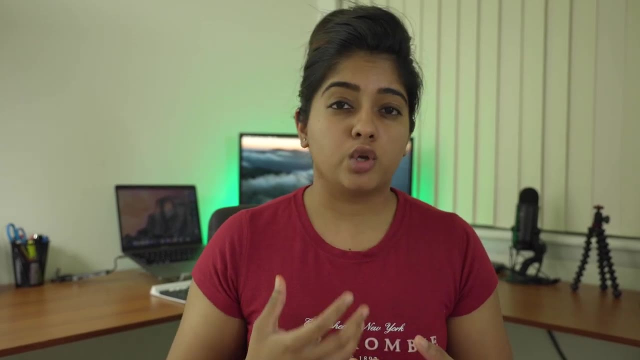 something called a lab-on-ship technology at Harvard and I thought that was really cool. So my interest like changed from that and now I wanted to do this. That stuck along for some more time and by the time I finished my undergrad I felt like I wasn't done. I wanted to know more. 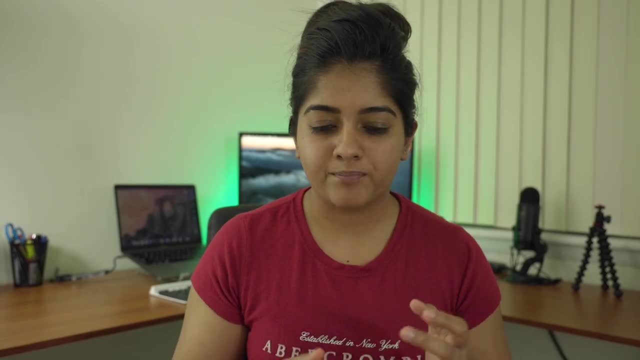 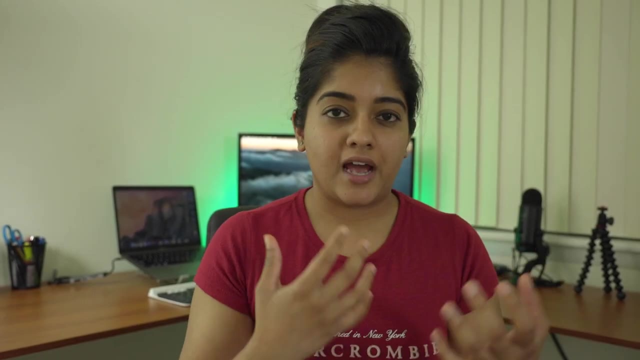 about this field that I kind of like left midway That led me to doing my master's in Cornell University. I continued to apply and learn more about how I can, you know, use my skills to develop this field of microfluidics and eventually that stuck around. 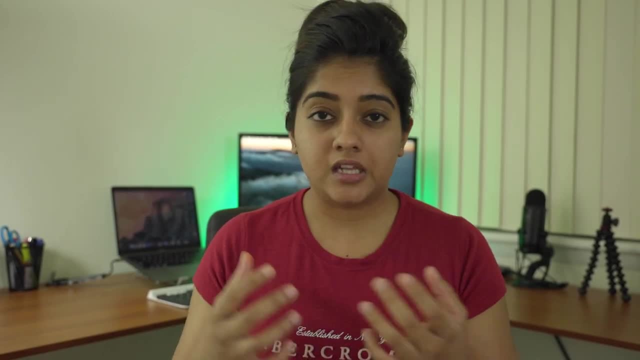 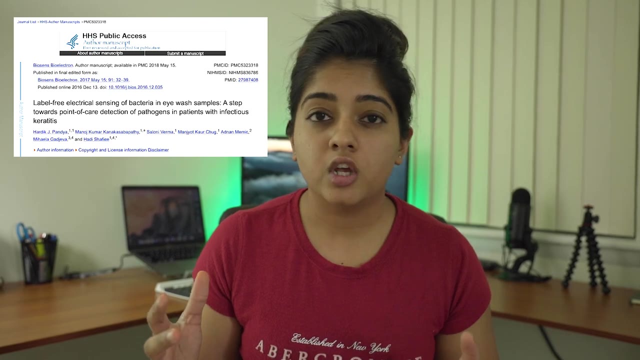 even further, and now I'm in a job which is basically lab-on-chip and microfluidics and I absolutely love it. I've gotten a paper published in a really high-impact journal when I was at Harvard Medical School, and this has just been all such a fulfilling. 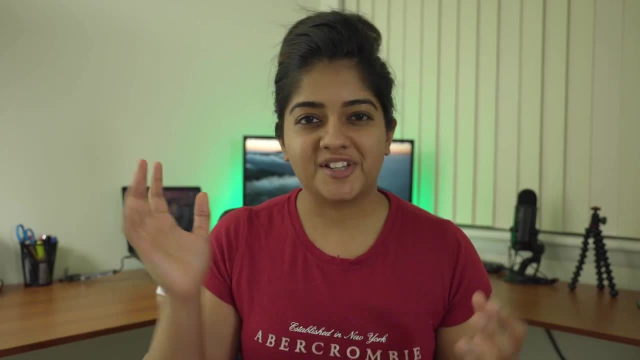 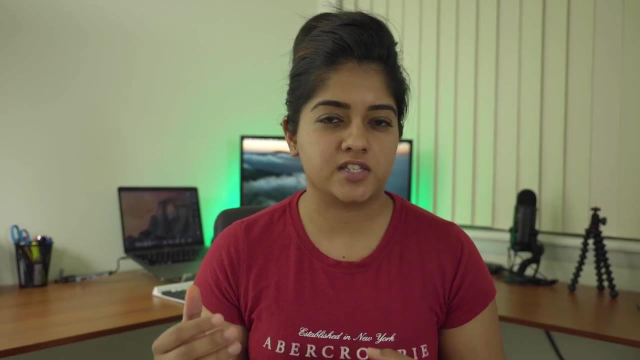 right to just do so many different things. So my point here, by telling you guys all this, is that it's okay if you don't know or you don't have it figured out, but you just know some pieces of it, you know. yeah, I think this is something I'm going to do. it might be fun to try. 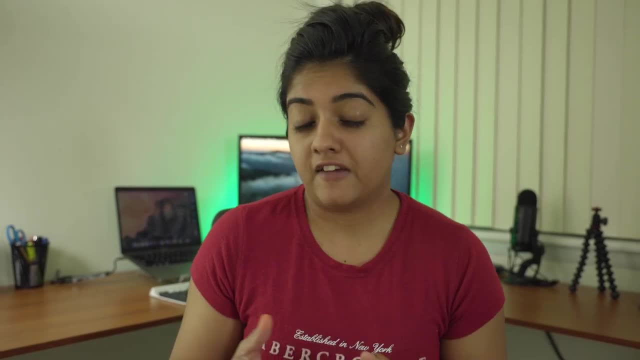 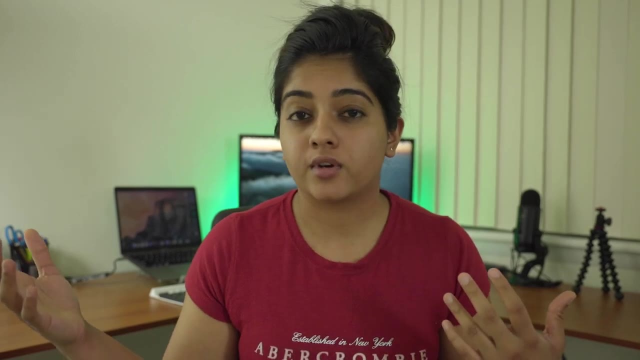 out. That's all the push and that's all the motivation that you need If you think you might be interested. the only way to be sure and to be firm on that decision is to try it out. That's all I'm going to say. It's okay to make mistakes, it's okay to fail, but just make sure. 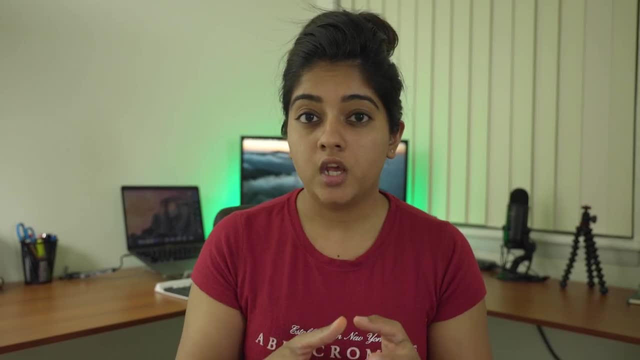 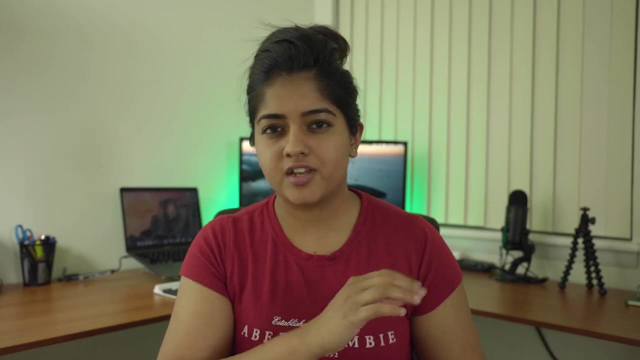 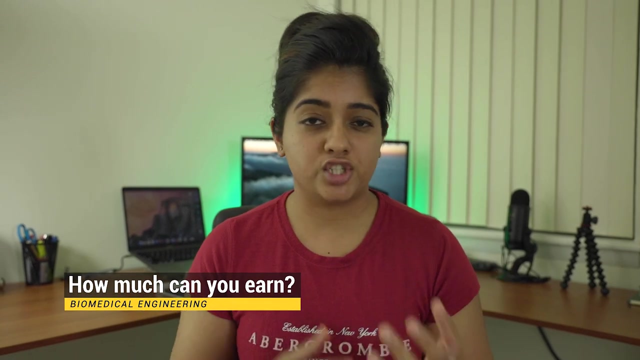 that, whatever you pick, you're putting your 100% effort in in making yourself better at that craft. Okay, so that's a lot of motivation and inspiration talk. Let's come down to the important stuff: Numbers. How much can you actually make with this biomedical engineering degree? 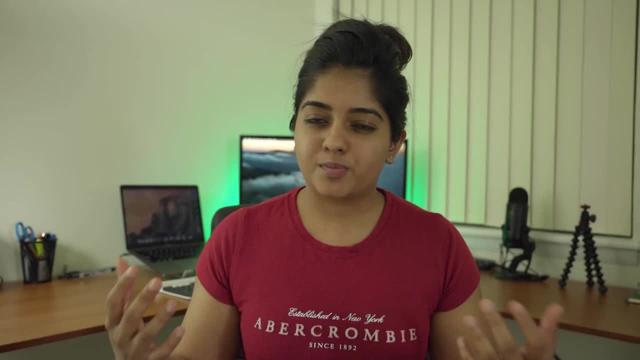 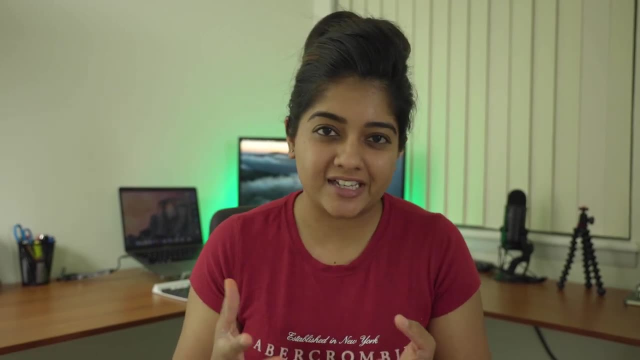 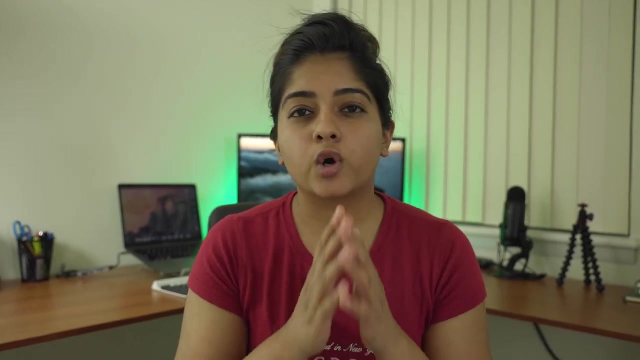 and what does your career look like? Now? come on spoiler alert. I bought a Mercedes at 26, so I'm just going to put it out there that it's a very promising career, finance wise, and you're not going going to fall short or regret this in terms of being financially independent. Now, according to, the US Department of Labor, the mean salary for a biomedical engineer revolves somewhere around $95,000 per year, with the top 15% earning about $150,000 per year. Now, I just want to point out that this whole category is very, very elaborate, because this involves fresh graduates as well as 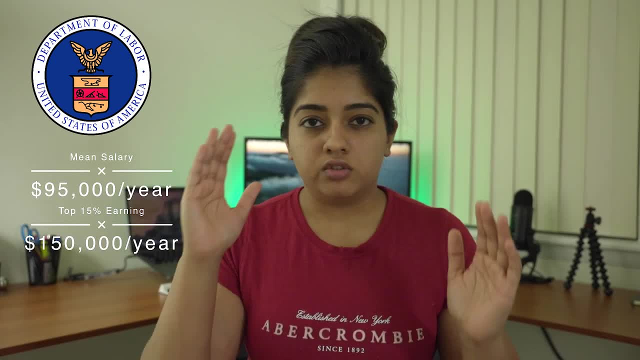 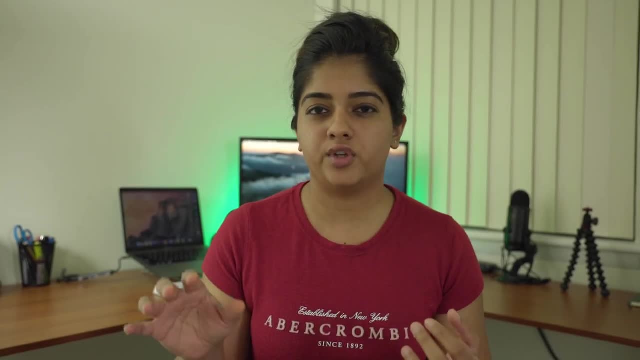 people who've had years and years of experience, So that's like a good range to have in mind when you're thinking of, you know, pursuing this degree. Now, economically speaking, let's treat this entire field like it's on the stock market. The diagnostic industry is currently tripling every year, which 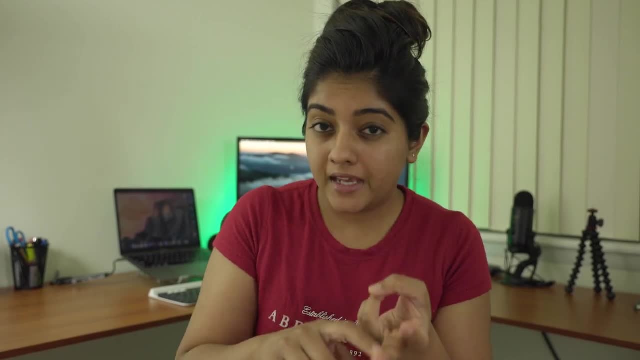 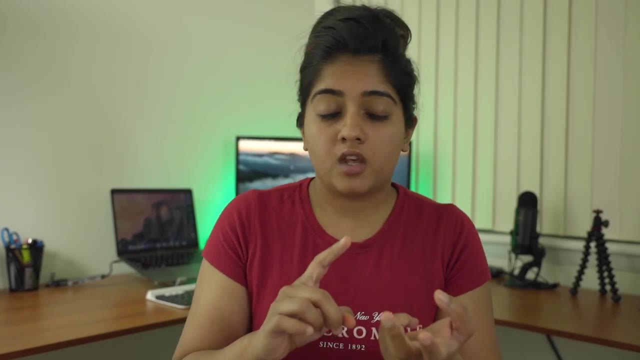 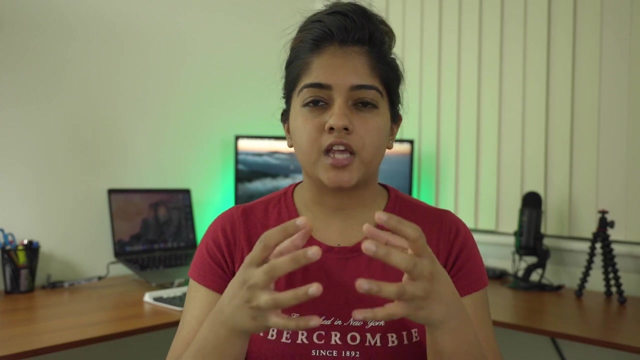 means that there are going to be more jobs. there are going to be more higher paying jobs, and the advancements that we make, like I mentioned before, by using the expertise of chemistry, physics, mechanical engineering, AI, the more and more we get all of this into healthcare, this area is just going to blow up. So, yeah, there you have it.